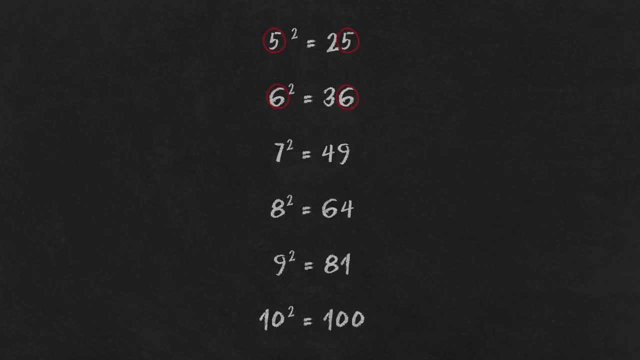 is just next to very round number 50 and 7 is otherwise 95.. 8 squared is 64.. 8,, 6,, 4 make this association with counting down even numbers, And 9 squared is 81.. Connect it with this: 9 is 8 plus 1. 81.. Okay, let's get to second then. Usually, 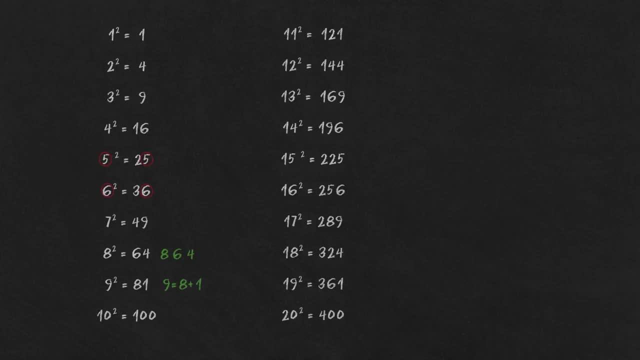 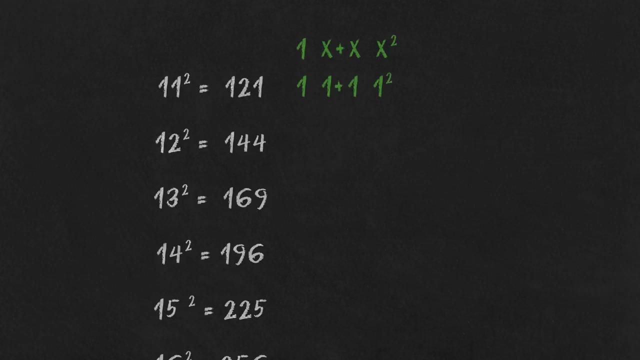 associations are made based on last digit of number squared. Notice that squares of numbers sharing last digit also have the same last digit, But three squares can be recalled from this basic pattern. It starts with 1, then double the digit, then square the digit Simple, And so 11 squared has a lot of ones, 1,, 1 plus 1, and 1 squared, 121.. 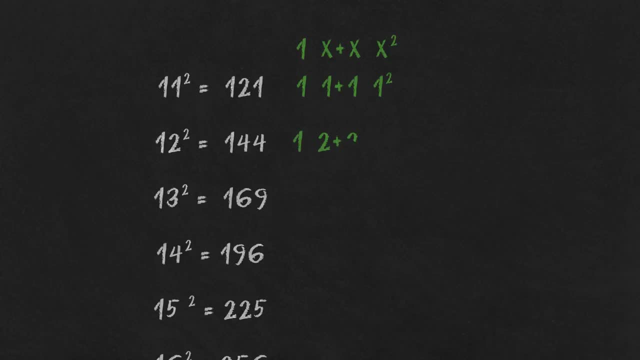 12 squared is 1,, 2 twos and 2 squared 144.. 13 squared is 1,, 3 plus 3, and 3 squared 169.. It's almost works for 14.. It would be 1, 4 plus 4, and 16.. So 196.. I think it's easier to remember previous. 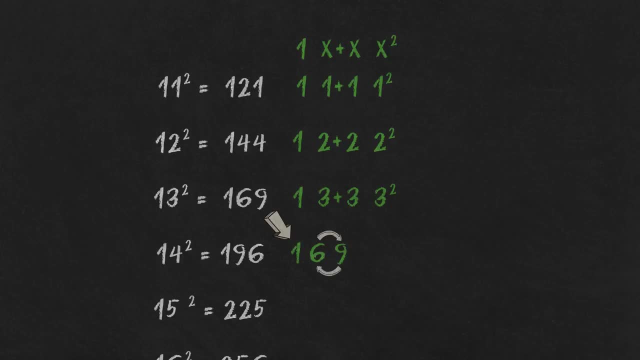 square 169 and the reverse order of digits 169 to 196.. Or you can remember that 14 squared is just 4 short of 200.. For some squares, as you see, I have a few ways to memorize it, So just pick one. 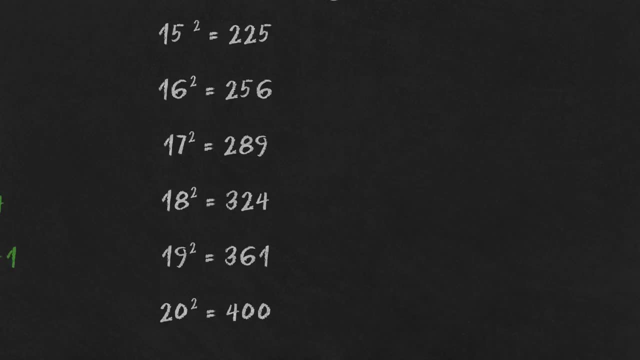 for yourself. Squares of numbers ending with 5 are easy. They always end with 25.. And we will talk about it more another time. 16 squared is the same as 2 to the power of 8. It's 256.. An important number in IT as byte is 256 bits. If it means nothing to you, 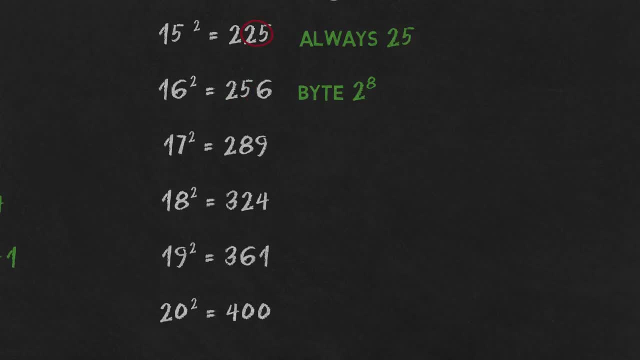 then maybe remember that this square starts same as previous square ends: 17 squared is 289.. 7,, 8, 9.. Easy to remember: 18 squared is 324.. 32 is an multiplication of 8. And so is 24.. But I remembered as this: 8 times 3 is 24.. 324.. Nice.